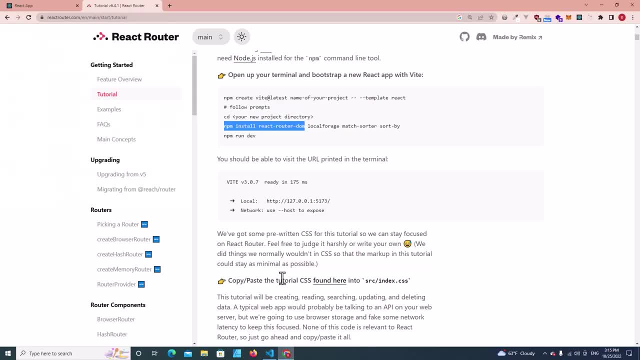 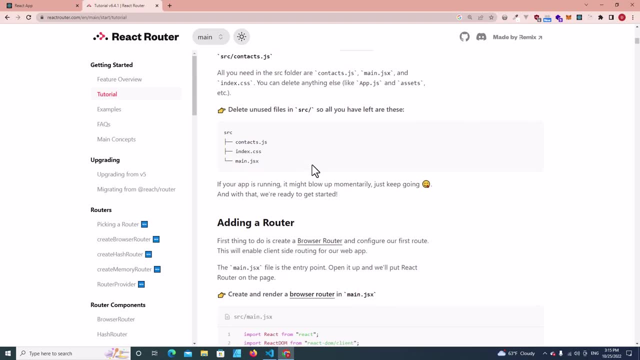 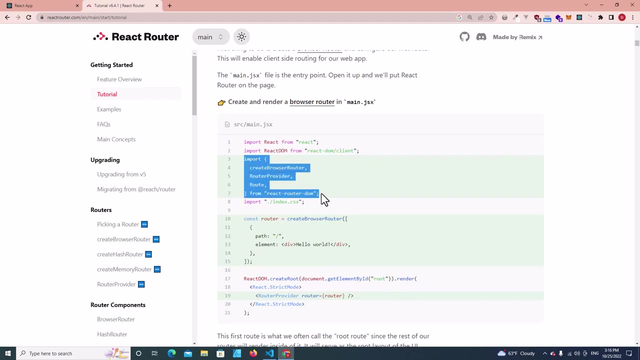 Let's go to indexjs over here and then go back to this tutorial. I have read this tutorial already, so I'm going to show you how to integrate React RouterDOM into React right now, So you just import these three components to your application from React RouterDOM. 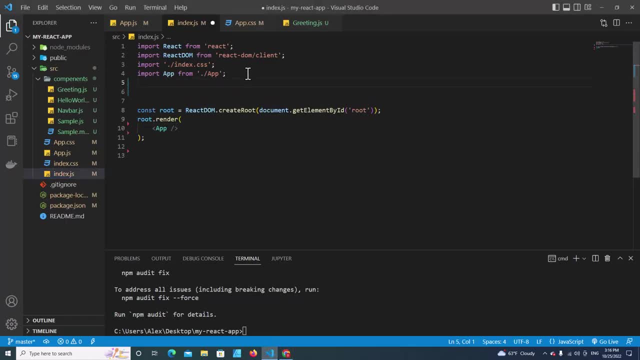 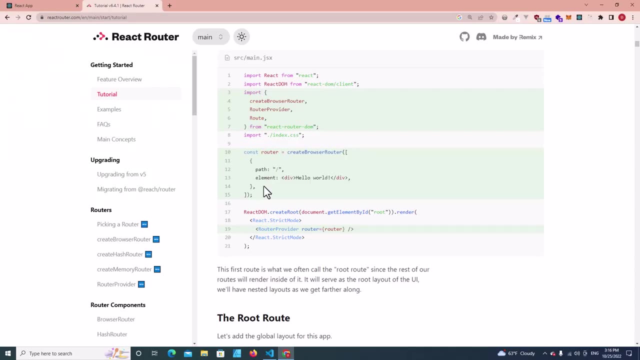 So copy this one, go back here and then paste this over here. The next thing you have to do is to create router to specify each route in your website by using create browser router. Copy this one, paste this over here. This create browser router is imported over here. 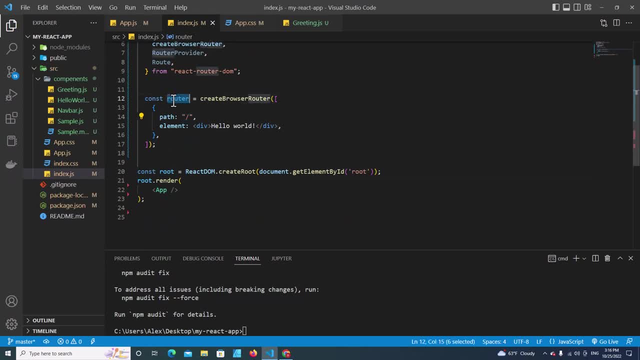 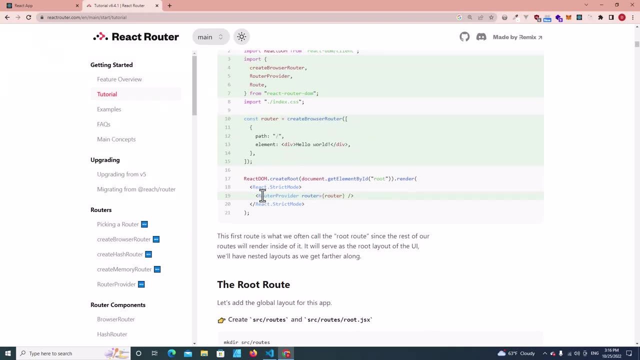 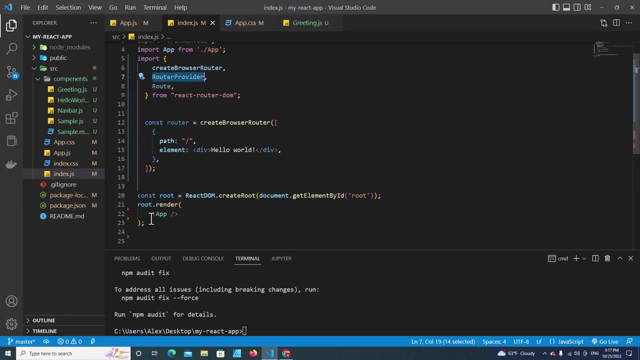 We get the first route over here, so we have to integrate this router to our application. Okay, what can we do? So we use router provider and then we include router inside. So we use this one. So I'm going to remove app over here. So then I'm going to use. 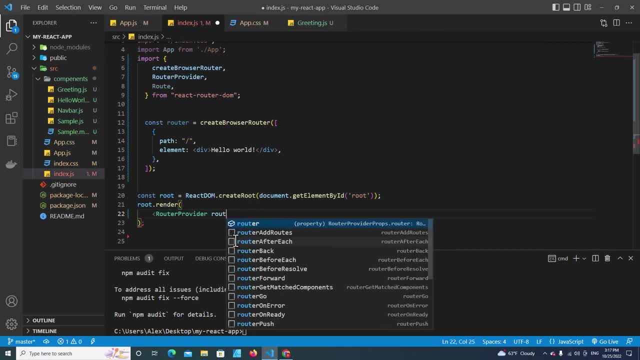 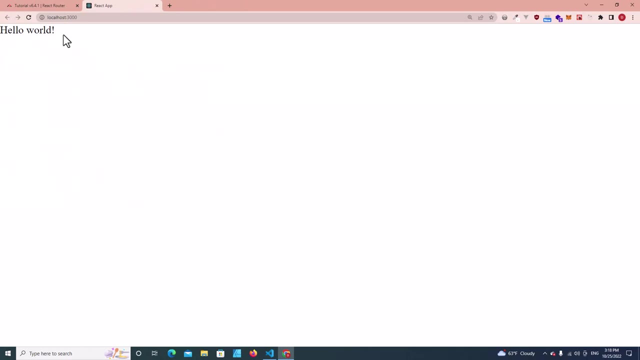 router provider and then we pass in router and we pass this router. Okay, we save. Okay, next we can run npm start. Okay, our application is running right now. When it's finished loading, you will see hello world over here. Hello world, is this one in our code? 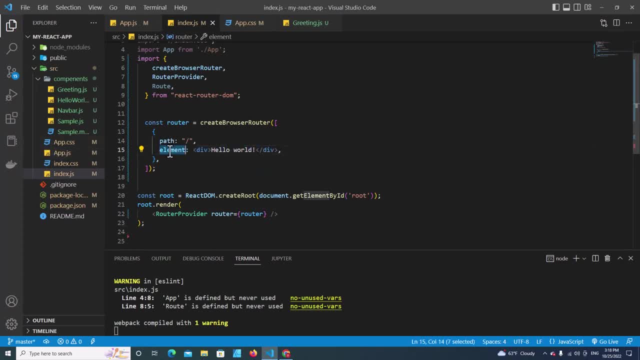 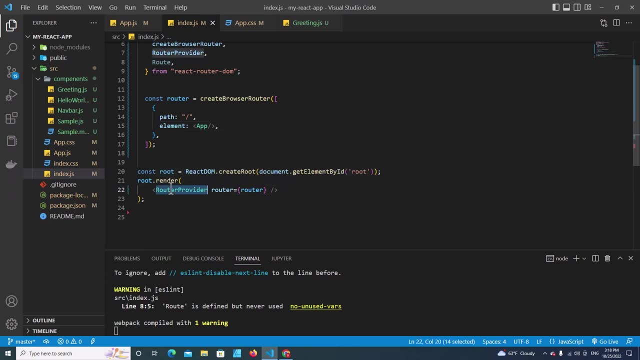 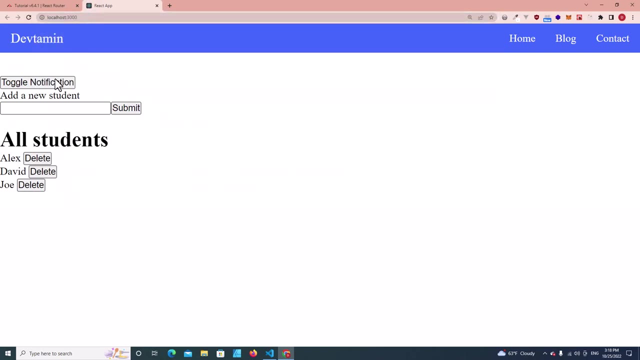 Okay, so how can include app in this one? So we just include app directly over here. Instead of put app over here, we move it in here. So this is the path which is the url over here. So this path, right, We get this one. 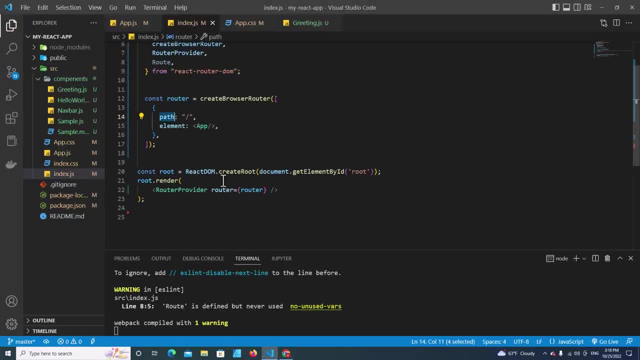 All right, so how about we create another pages? So I'm going to create a folder over here, inside source I create new folder and name is pages. Okay, and inside here I can create block page blockjs. Okay, I have see it enter. 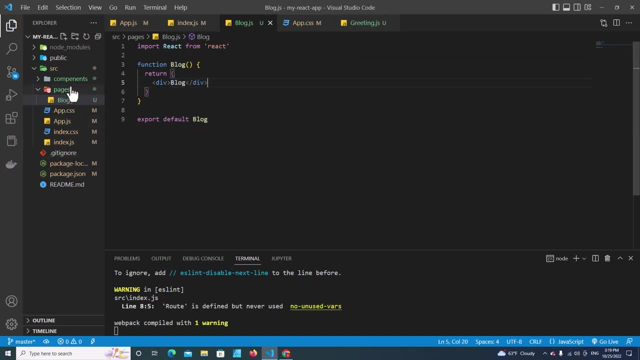 I have block component over here So I can include a nav bar over here. So let me import nav bar component. Okay, we have nav bar component. All right, then we include nav bar over here And here we can create div and then we put block page. Okay, save. 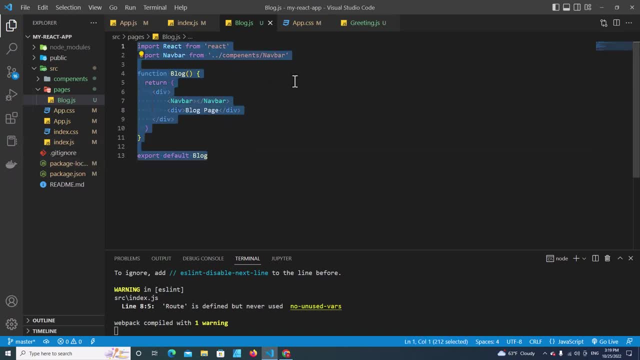 Okay, right now we get this page, but this page is not in our application yet. We have to integrate this over here, So we have to specify the path. copy this one put here: The path is block. right, Okay, and the component that we want to load when the user access this url. We want to load block. 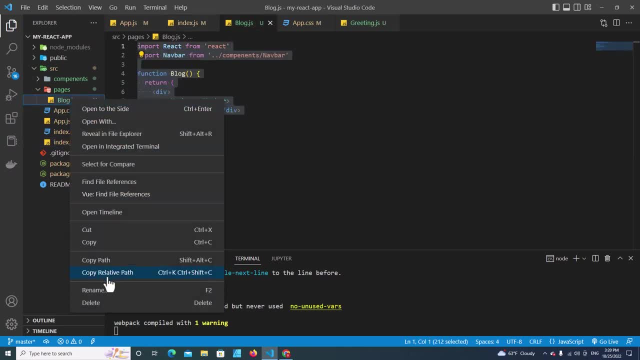 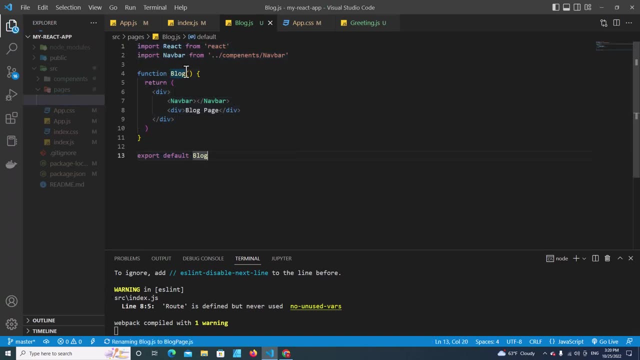 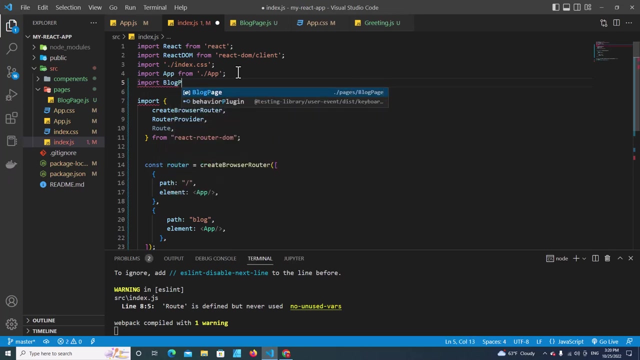 page, which is here. Let me change this one to block page. block page: Okay, and this one. I'm going to change this one to block page page and go back to index. we have to import a block page. import blog page. okay, then we load blog page over here. so when we access this url, it's going to. 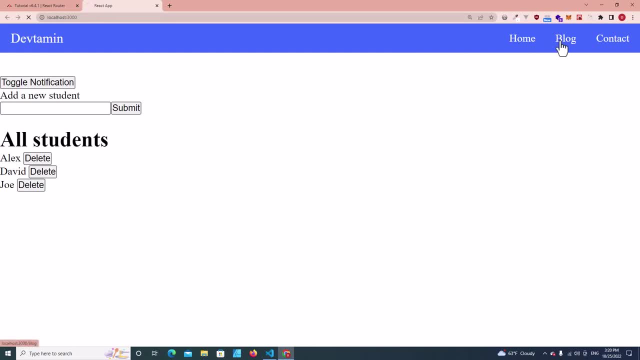 load this component. click on blog over here. see, we got blog page. or we can enter url directly if we click on home. but you see that this is not a single page application, because every time we click on the link is refresh the page. so how can we stop it to refresh the page? so we have to use 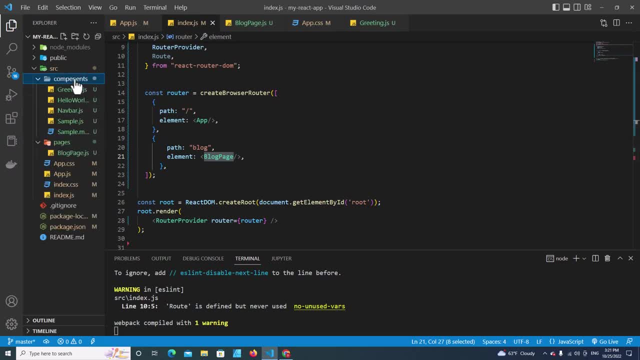 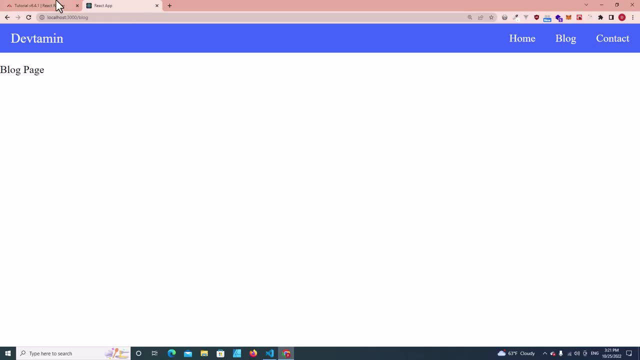 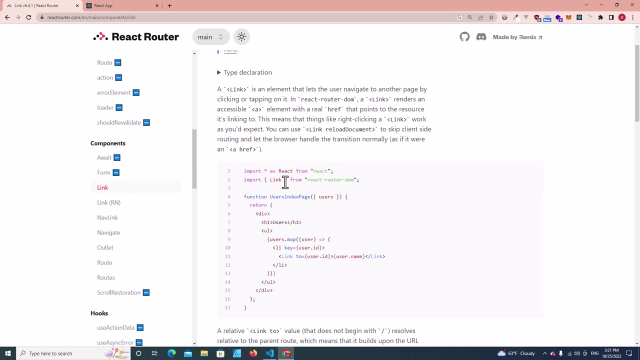 link instead of a tag or angle tag. okay, we go to component and we go to navbar. you will see we use a tag. right now we have to use link. so where can i get link? uh, link is over here. it's component link. it's come with react router so we can import it like this. so we copy it. 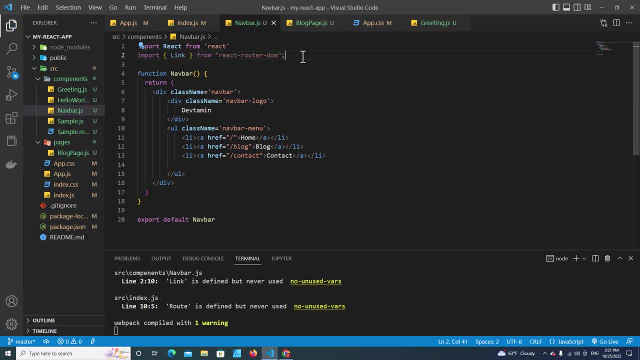 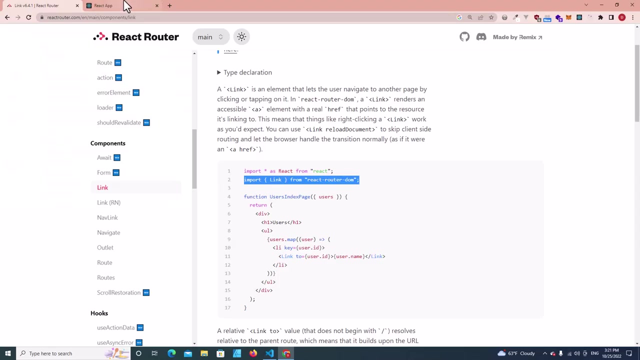 paste it over here or you can type it directly over here. import link from react router dome. so how to use it? we remove this one, so we call it link and then we put blog over here. this is what show on the website, but this is the path we link is to blog. okay, when we go back here, if i go to 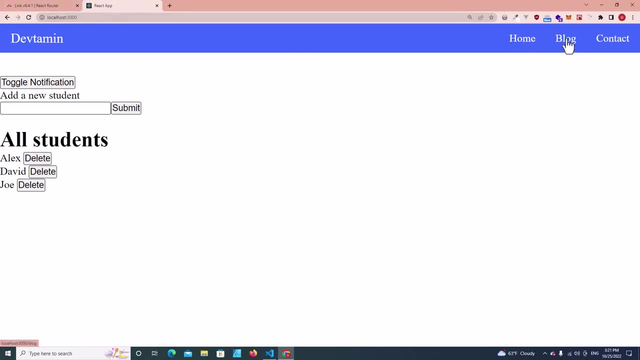 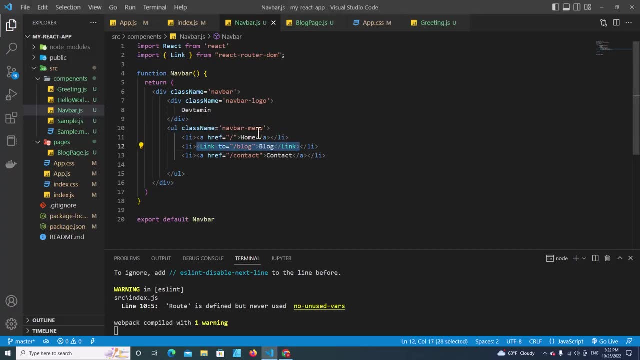 home, it still refresh the page. but if i go to blog it doesn't refresh the page. so we have to change home as well. so just copy this one and put this over here. so i put like this and put home over here, save, and when i click home here, see, this doesn't refresh the. 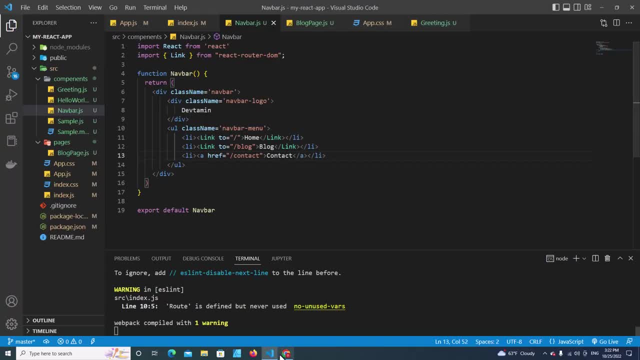 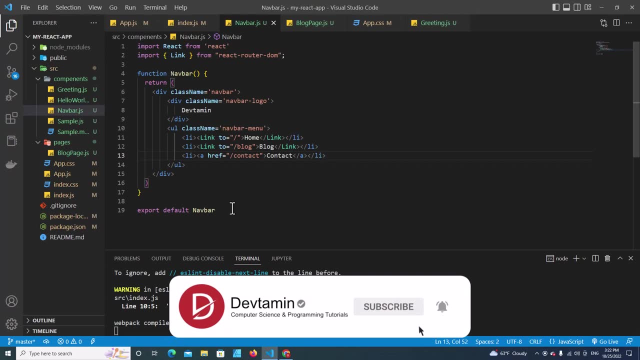 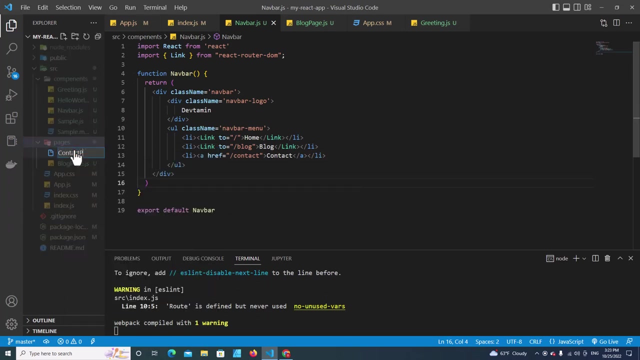 page anymore. so how about contact page? how can i create contact page right now? we have set up everything completely. creating other pages. it's going to be very easy. for example, i go to pages, right click new contact page. okay, i have ce, hit enter and we can copy this one, okay. 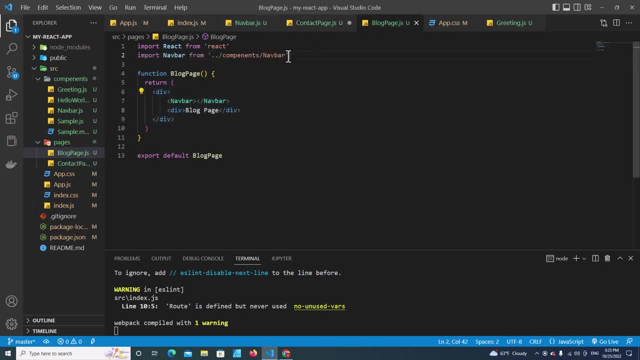 but it's like this and we have to import navbar as well. put navbar over here. this is going to be contact. okay, we get contact page. don't forget, we have to add this page into indexjs. copy this one, paste this over here, then put contact. okay, import contact page over here. import contact page. 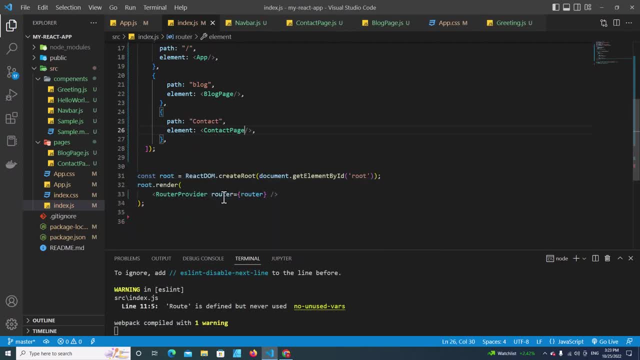 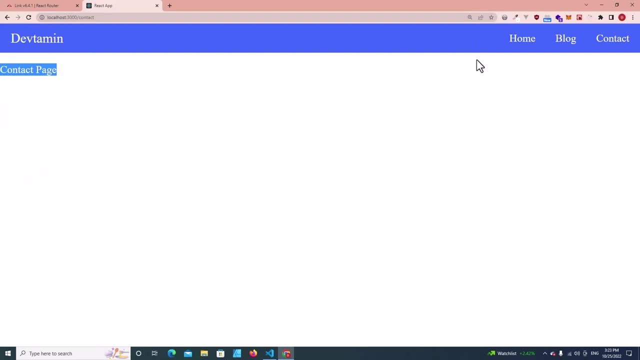 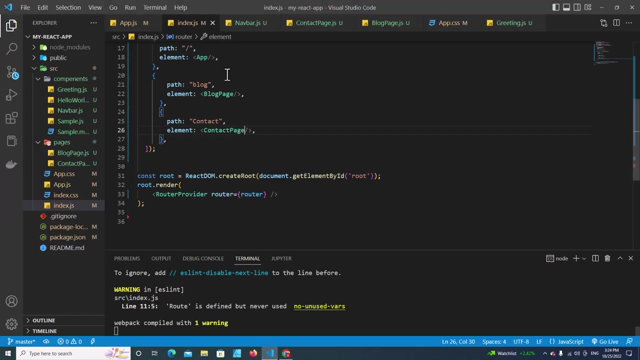 and then load contact page over here. okay, save. so if you go here, we type contact. so it's load contact page. all right, what next? we have to change this uh link. right, because right now it's just anchor tag. let's go to navbar, remove this one, copy this one and put contact over here. this is going to. 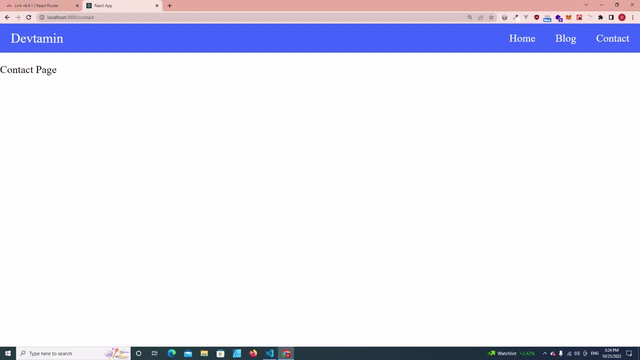 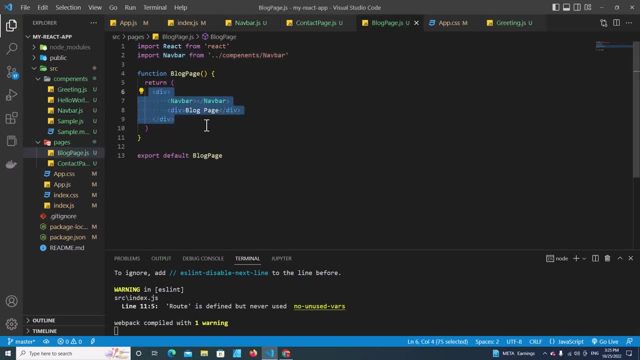 be contact save. okay, you can see it works perfectly. all right, what's next? i can do? as you can see here, the code over here is repetitive. you see blog page. the code is almost the same. so how can we reduce the code? we are going to use layout, so let me create. 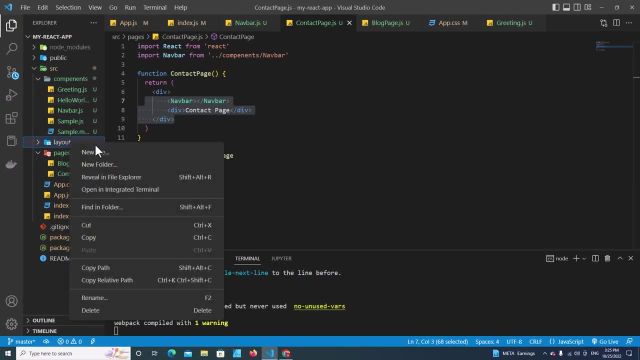 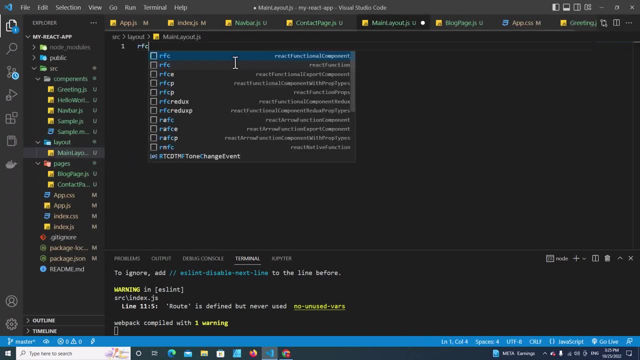 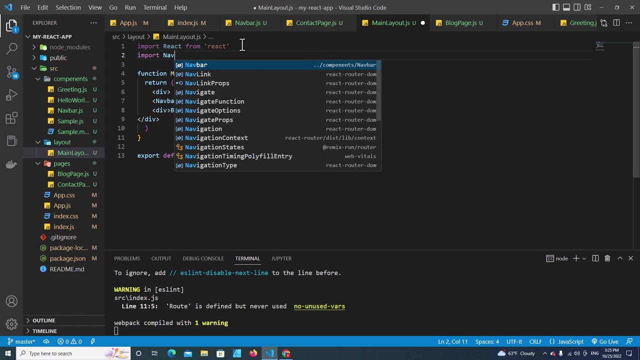 layout folder over here, layout, so i can create here new main layout dot js, so rfc. okay, i can copy the layout from here. just copy this one. put this over here and we have to import navbar. okay, let me format document. okay, and this one is where the content appear. okay, instead of. 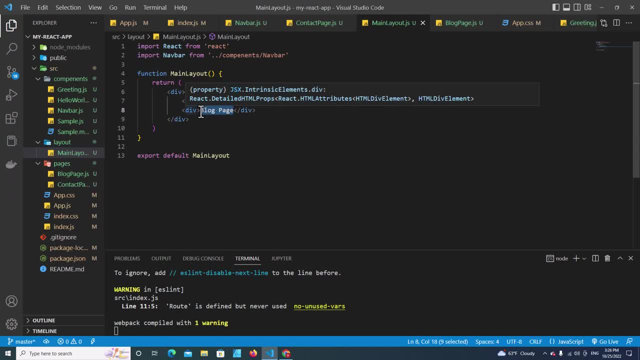 put content directly in this div. in main layout we put children- okay, curry base children- and over here we put children in parameter in function. okay, it's going to be like this: we are going to pass children and show children over here in blog page. instead of coding like this, we are going to import main layout, okay. 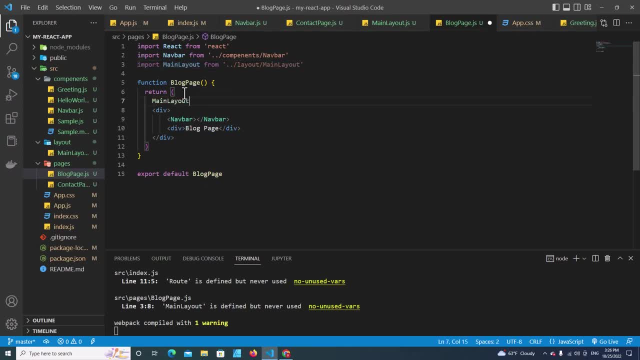 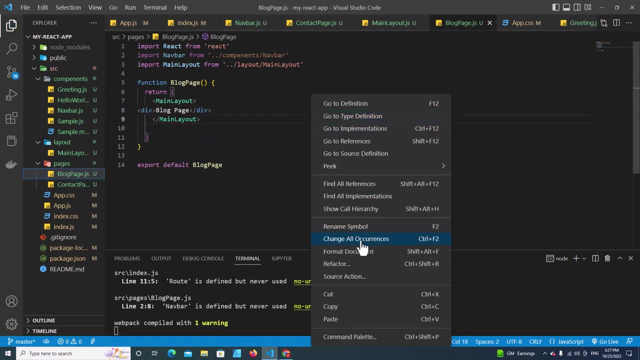 and we can use main layout as a parent layout, as a parent component. okay, main layout. then we pass children, which is information that we want to show inside main layout in children over here. okay, we pass this div inside here and remove this one. let's format document: okay, it's going to be like this and if you go to contact 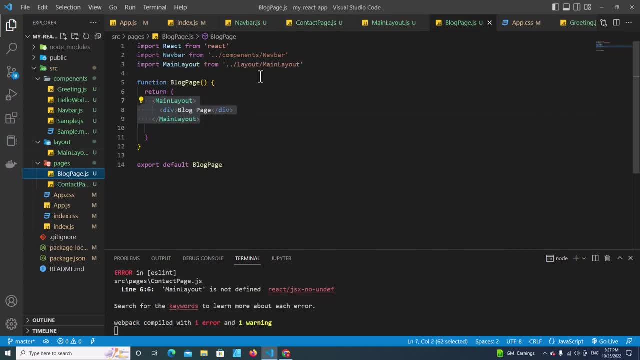 you do the same, but you have to import main layout. let me copy main layout over here, so we don't need a navbar inside blog page anymore. we can remove it and this one just import main layout and this one needs to be contact. let's format document. it's warning that route is defined but never used. we can remove. 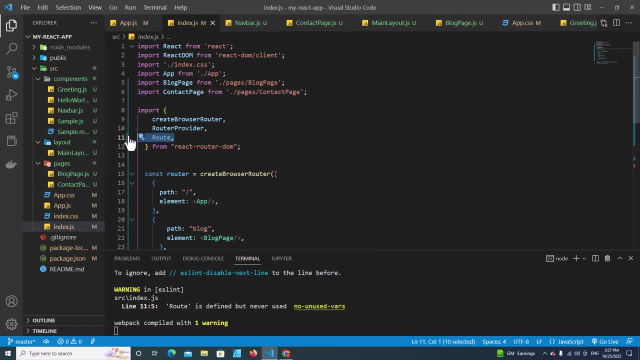 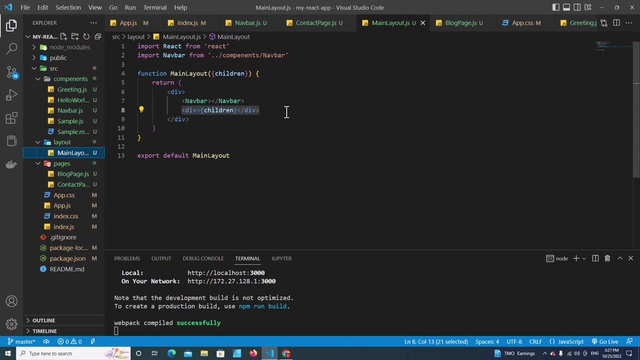 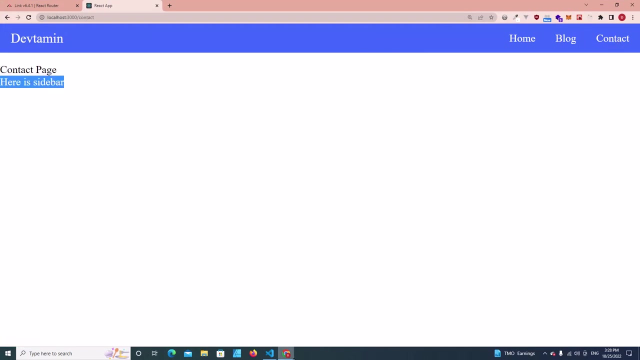 route from here here. okay, let's go back here. see, it's work the same, but we have layout over here, so if we change anything in layout, every page is going to change. for example, if I want to add sidebar, if here is sidebar, okay, you can see that blog page has sidebar and contact page has sidebar. you can even 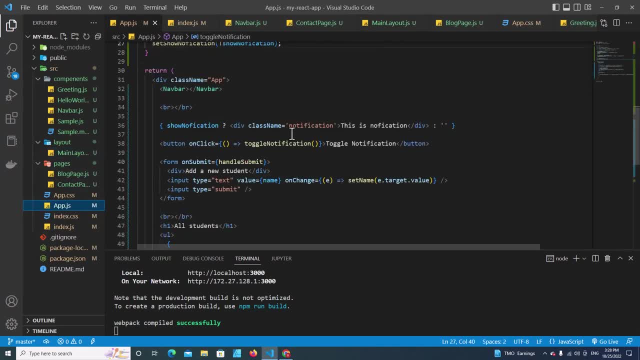 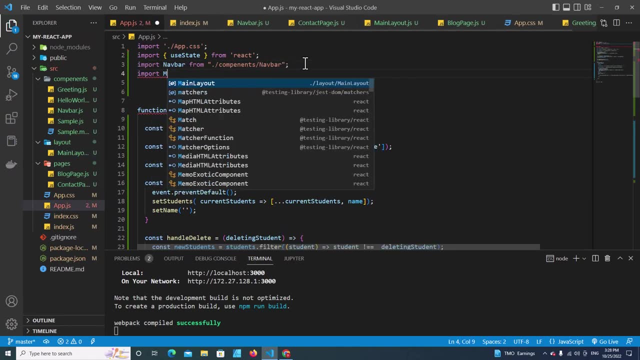 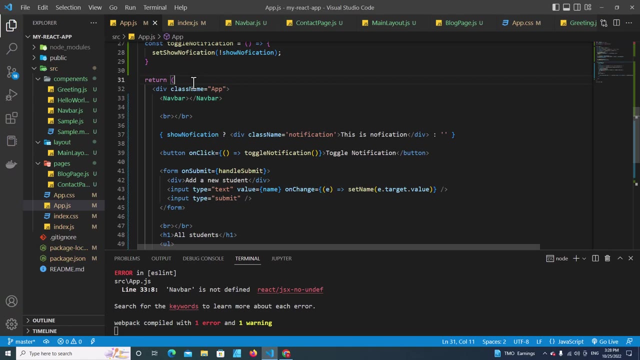 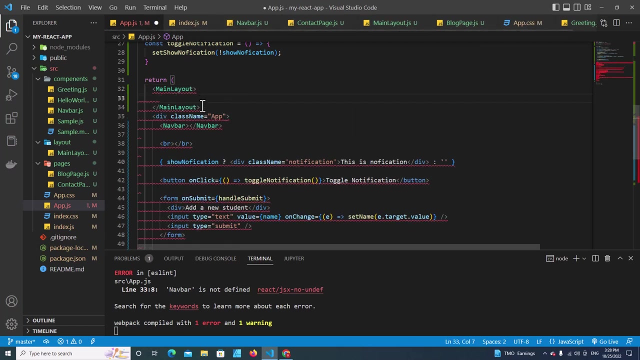 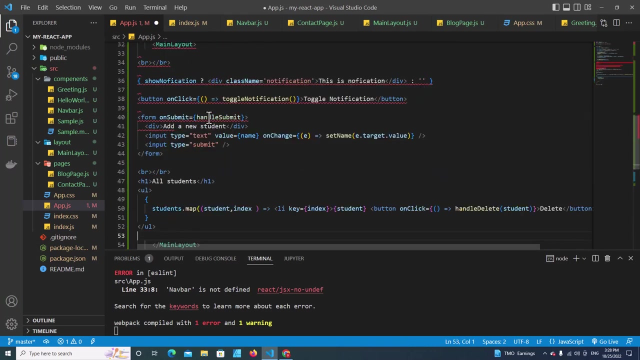 use this main layout. in have touches as well. it's going to be the same. just import main layout. okay, you can remove navbar over here and over here we can use main layout as a parent layout. okay, main layout. okay. then we copy all content over here, cut it, paste it over here and we can remove this one. okay, let's format.